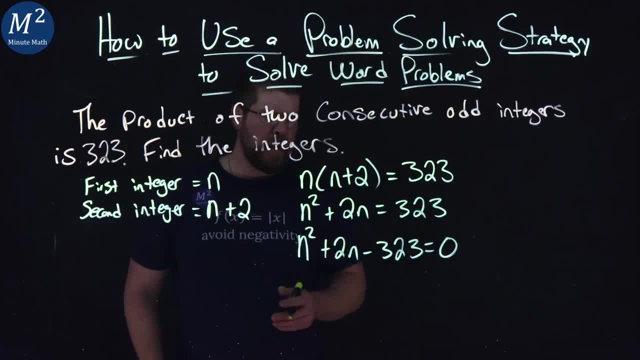 and that equals well 0.. Now I can solve this quadratic in many ways, but I'm going to solve it by factoring Right here: an n equals 0.. What two numbers multiply to be negative 323, but add to be a 2n. 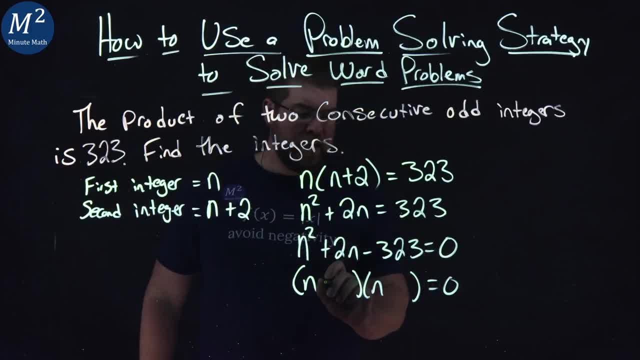 I know off the top of my head, hence I've also looked at this problem. Negative 17 and a positive 19.. 17 times 19 is 323, or specifically a negative 17 times a positive 19.. But they add together to be a positive 2.. 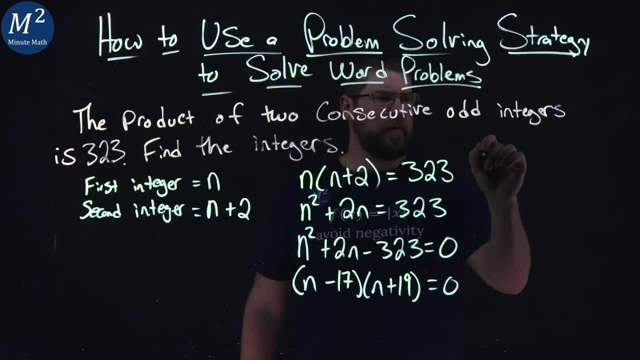 From there we solve each one individually, which we can do up here. n minus 17 equals 0.. n equals a positive 17.. An n plus a 19 equals 0.. An n equals subtract both sides by 19, negative 19.. 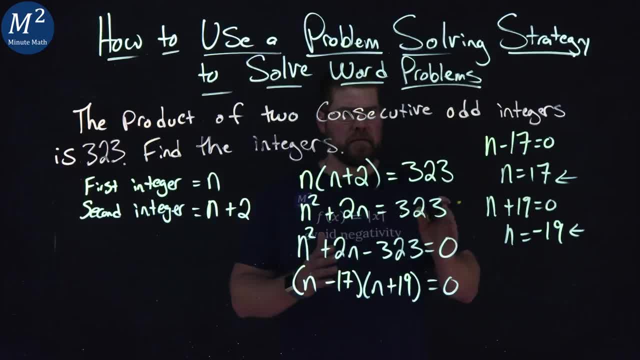 So these are the two values we want to work with. Notice, it's not. these aren't our answers here. okay, This is what possibly n could be. Now they would be consecutive odd integers, so let's go test that out. 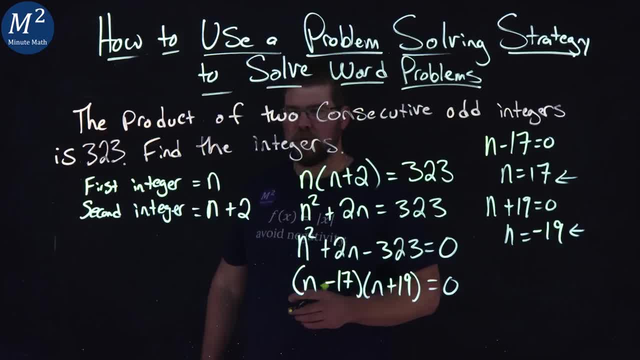 n equals a 17,. right, Let's go test that first one out. If n equals a 17, that means the next integer consecutive odd integer would be 19.. So 17 times a 19, what does that equal? 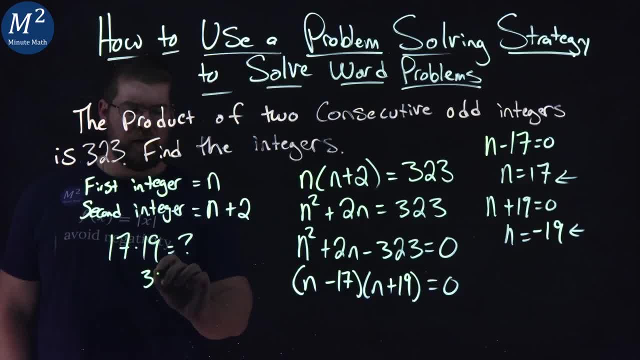 Well, we kind of already know: 17 times 19 is a 323.. So 17 times 19 works here, it's a 320.. So 17 times 19 is a 323.. Now what about the second one? n is equal to a negative 19.. 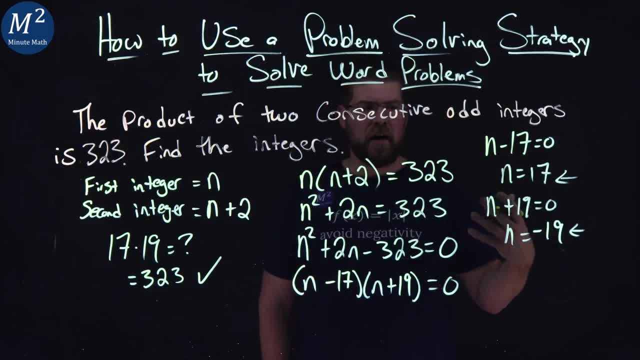 Well, if I put a negative 19 here, the next consecutive odd integer would be a negative 17,. right, So the first one is negative 19 times the next consecutive odd integer negative 17.. Negative 19 times negative 17,: what does that equal? 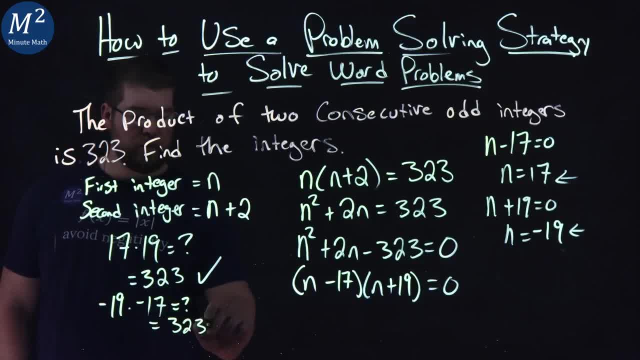 Well, a positive 303.. So we have two solutions here, two consecutive odd integers. The first one, 17 and 19.. The next one also works as negative 19 and negative 17.. Both of them are consecutive odd integer pairs. and well, they multiply together to be 323. 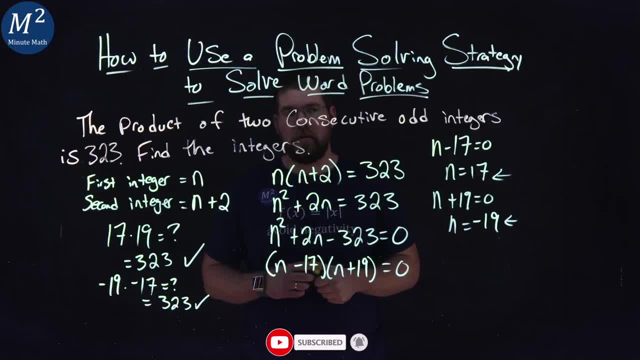 Hope you learned something here on how to use a problem-solving strategy to solve word problems. If you did, make sure you like this video and subscribe to our YouTube channel. This helps us make more of these free math lessons For you and for everyone else. So, as always, thanks for watching. 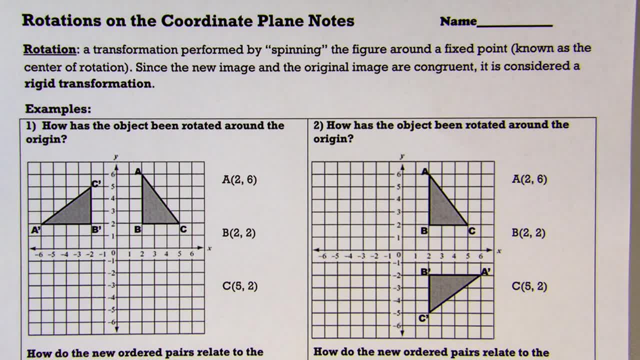 Alright, today's lesson is on rotation on a coordinate plane, So let's first start off with our definition of rotation. It's a transformation performed by spinning the figure around a fixed point known as the center of rotation And our fixed point in these. 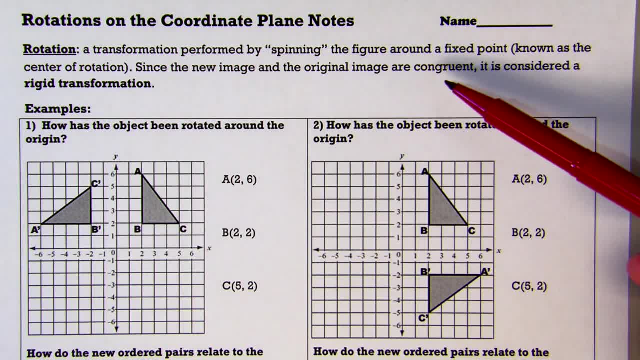 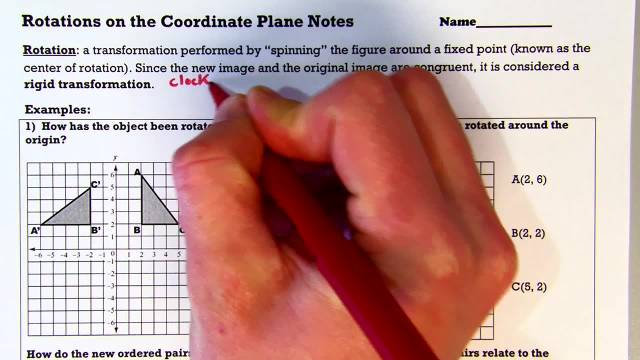 cases, is going to be our origin, our, Since the new image and the original image are congruent. it is considered a rigid transformation, So our shape is not going to change when we do these Now, we can rotate two different ways. The first way we can rotate is clockwise. 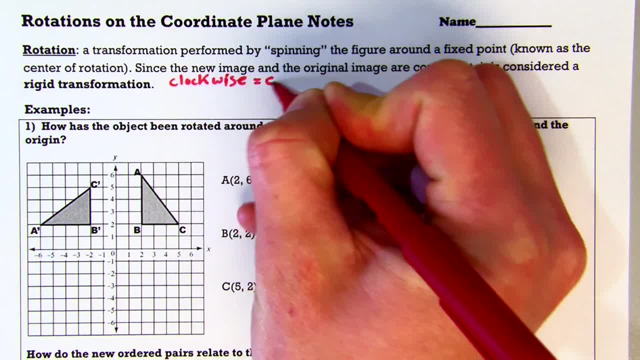 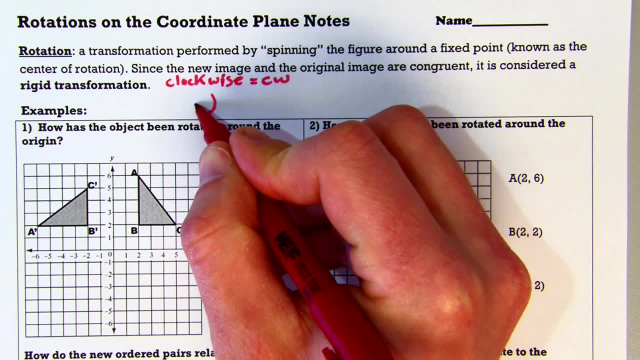 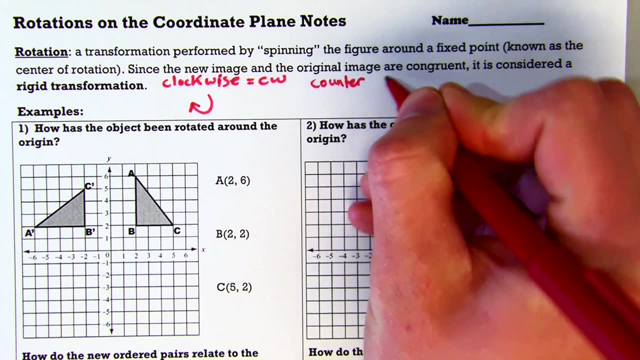 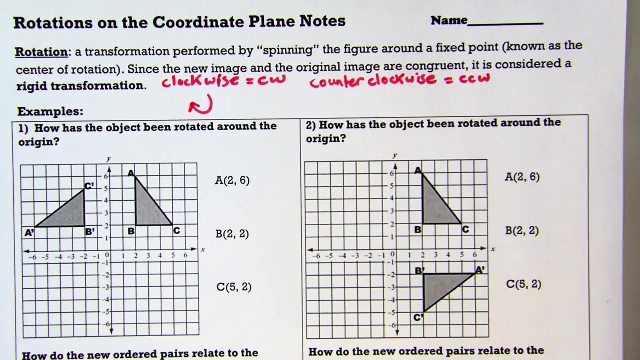 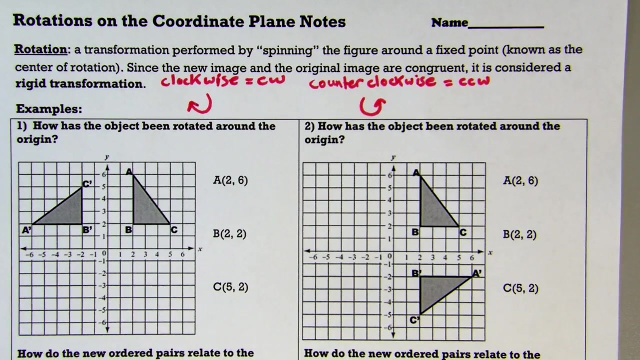 We're going to make that equal to CW, clockwise, And that is the direction that a clock goes. So that is this way. Another way we can go ahead and rotate is counterclockwise. We're going to make that CCW, And that is the opposite way that a clock goes. And in these examples, 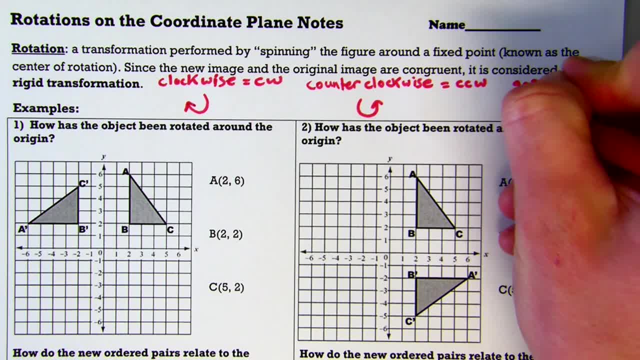 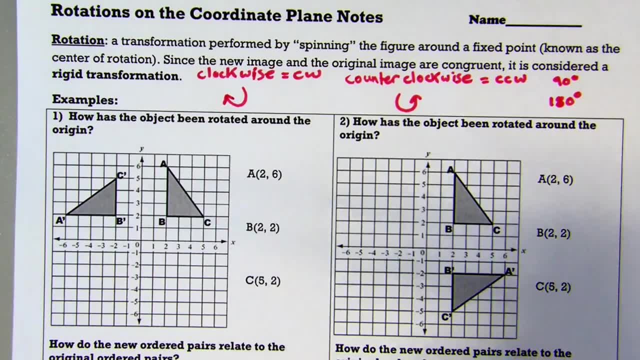 we're going to go ahead and rotate either 90 degrees or 180 degrees. Now, when we rotate 90 degrees or 180 degrees, if we look at our graph here, that means if we look at our graph- we have four quadrants: One, two, three, four. Whenever you rotate 90 degrees, you rotate. 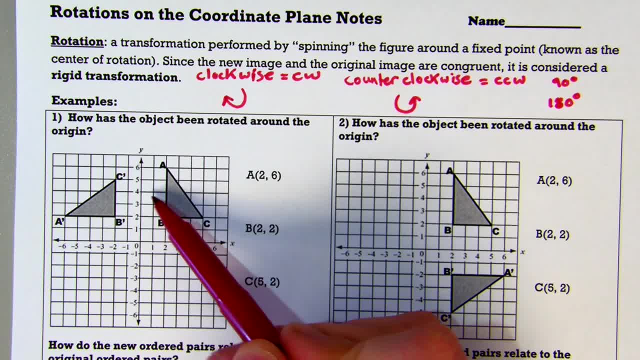 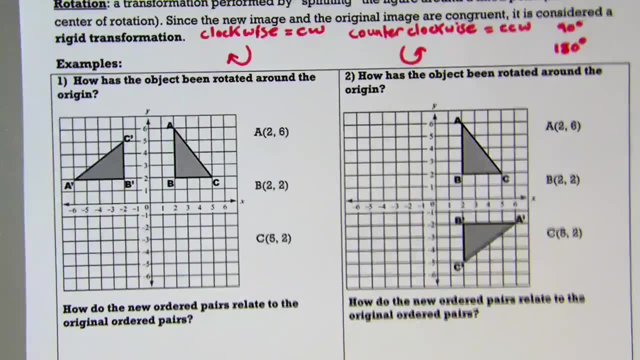 over one quadrant. Whenever you rotate 180 degrees, you rotate over one quadrant. Whenever you rotate 180 degrees, you rotate over two quadrants. So we're going to use those to figure these out. So our first example here, number one we have. how has the object been?